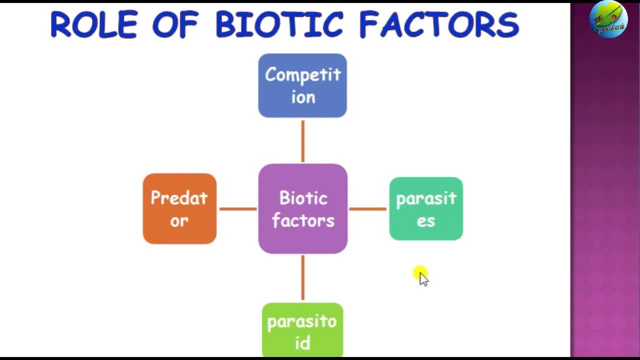 that is responsible for the fluctuation of the population. first one is competition. for at least part of a lifetime, the members of an insect species are likely to be competing with one another or with the members of another species for the limited resources, like food maids, suitable site. 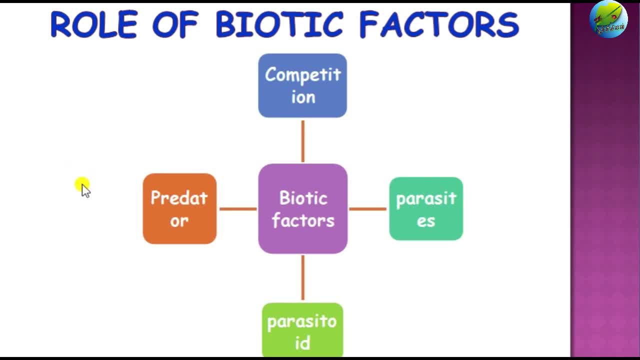 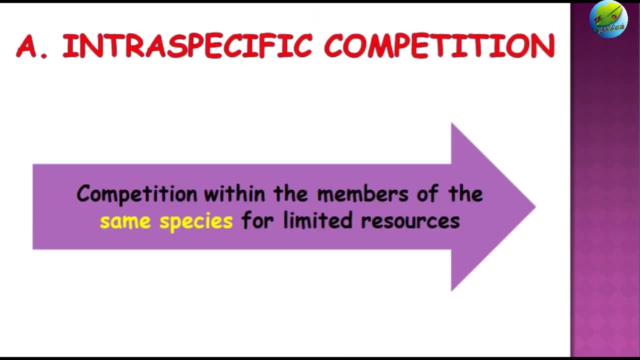 for oviposition or pupation. such competitions operates whenever the population is increasing and the resources are limited. there are two types of competition. first one is the intraspecific competition. that means the competition within the members of the same species for the limited resources. example of such 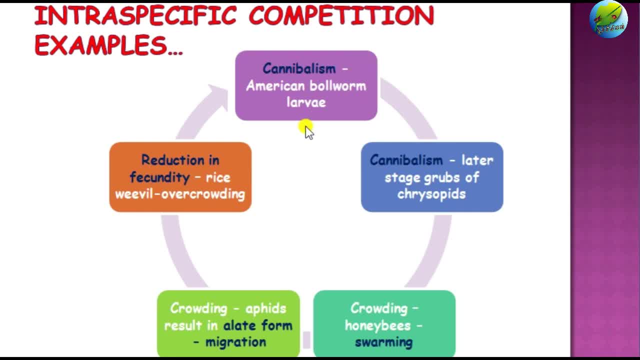 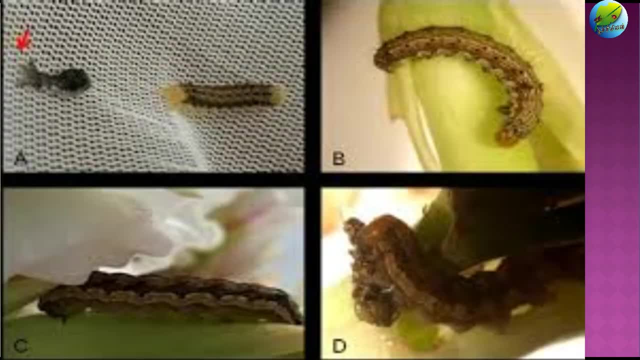 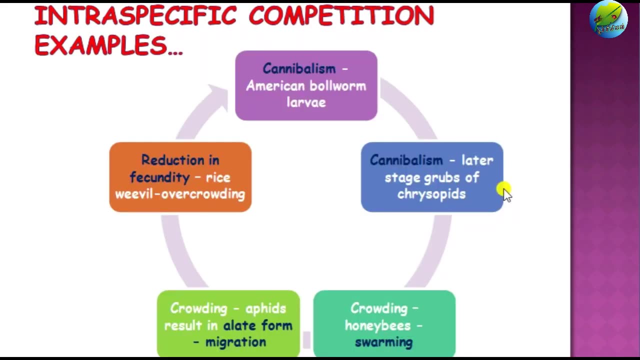 interesting intraspecific competitions are the cannibalism in case of American bullworm, if we see when there is a population, is more the larvas of the American bullworms feed on each other. she's called as the cannibalism and the cannibalism happens in the latter stage grub of chrysophytes, as these latter 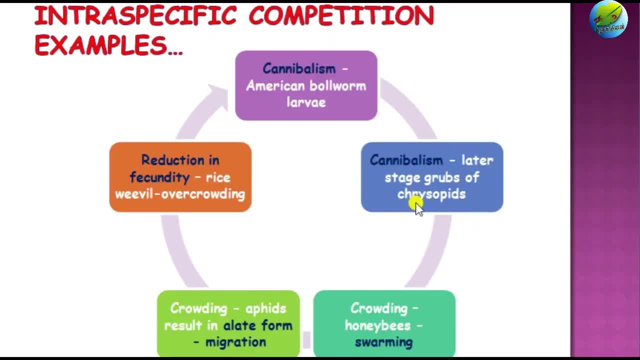 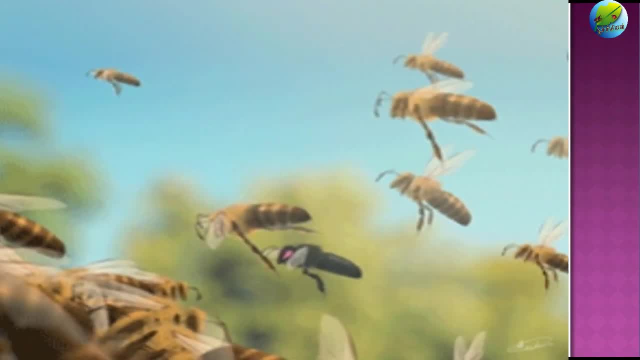 stage grub of the chrysophytes, they feed on their own eggs. in case of the honeybees, when there is a overcrowd, the population tend to swarm from one place to another, and in case of aphids, when there is a crowd, it results. 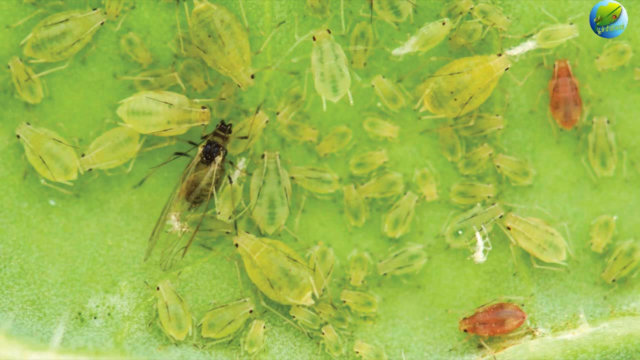 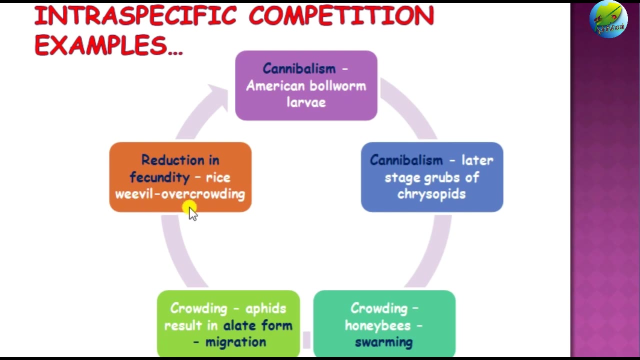 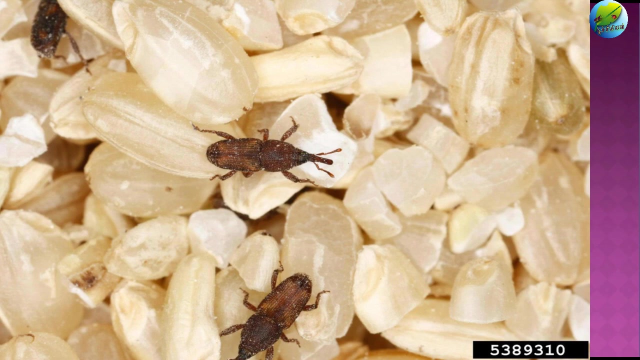 in the formation of the allied form or the winged form and which will be leading them to migrate from one place to another. and in case of the rice, we will. when the population is more and the overcrowding happen, the fecundity rate or the egg-laying capacity decreases, by which the intraspecific competition is. 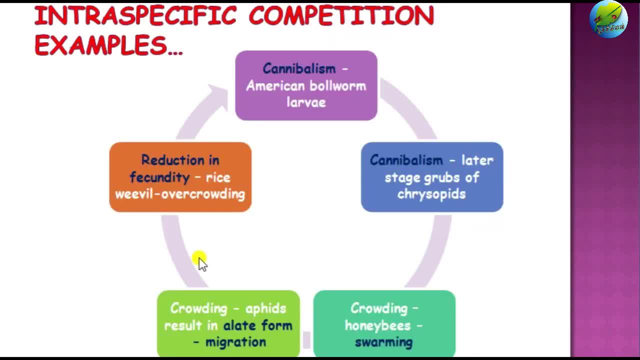 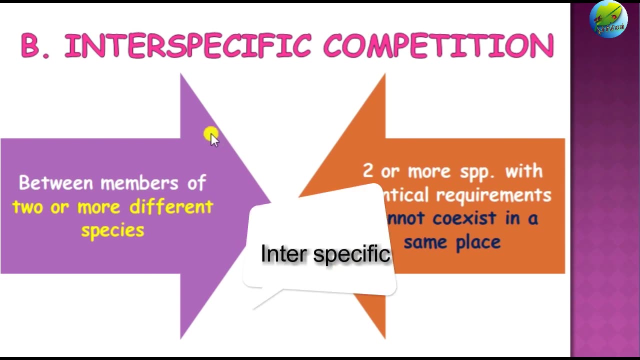 avoided. these are all the ways how the environment finds its balance order to avoid the population growing above the carrying capacity of the environment. the second kind of competition is the intraspecific competition. this is the competition occurring between the members of two or more species, two or more competing species with identical. 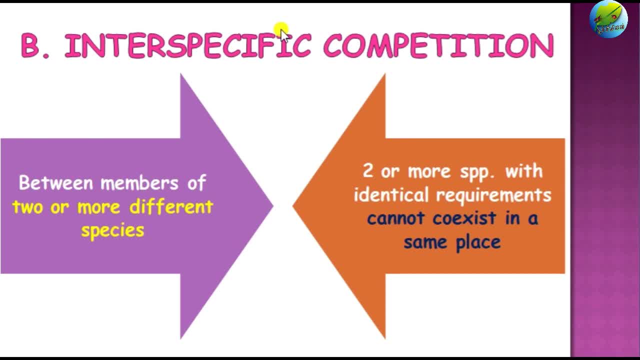 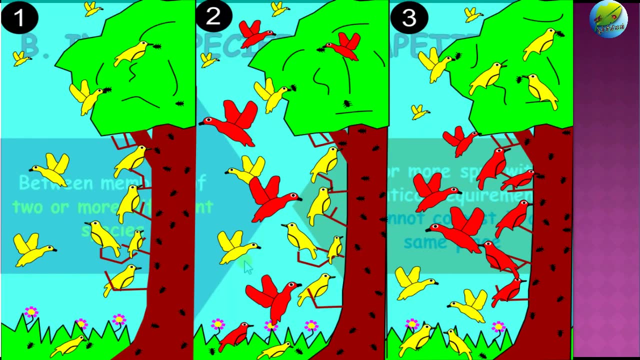 requirements cannot coexist in the same place. for a long time, the elimination of one species by another as a result of intraspecific competition has come to be known as the competitive exclusion principle of Gauss principle, which denotes that the two or more species with the identical requirements 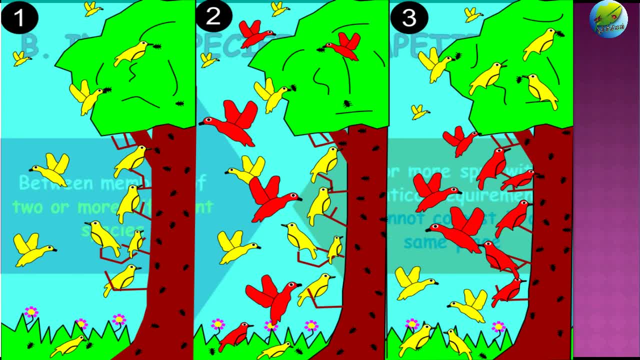 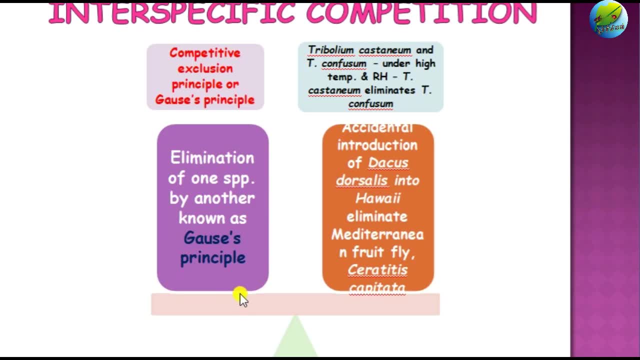 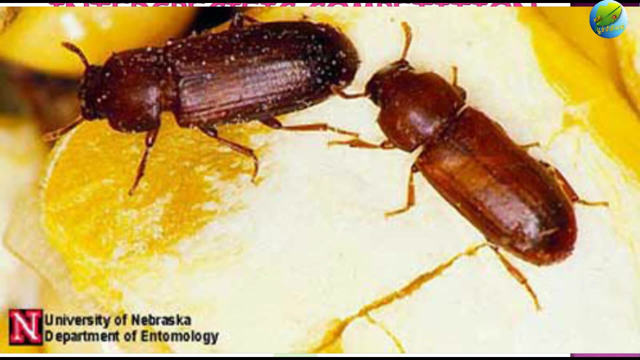 cannot coexist in the same place. for example, when the floor beetles tribolium castinium and the tribolium confusum were grown in the same jar of floor, one species eliminates the other under high temperature and relative humidity condition. tribolium castinium eliminates. 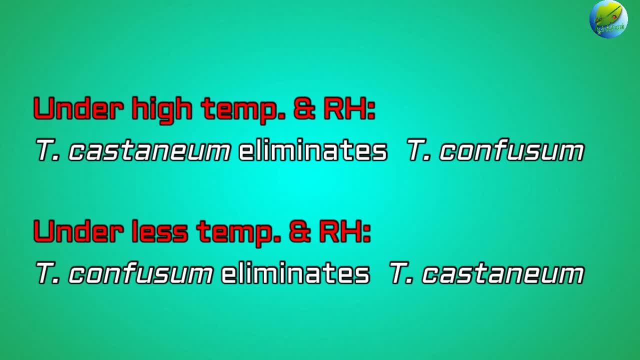 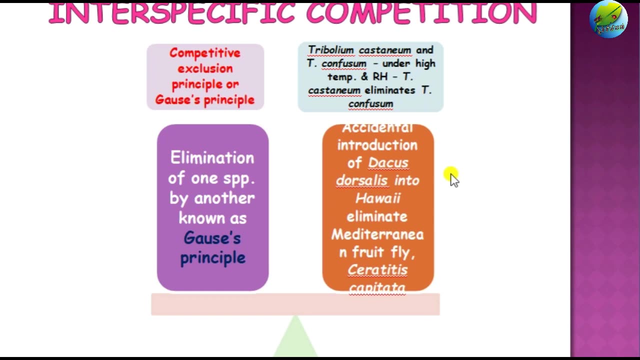 the tribolium confusum and vice versa, under the low temperature and relative humidity conditions, when the tribolium confusum will be eliminating tribolium castinium. and the another example is when the introduction of oriental fly, that is, Marcus dorsalis is accidentally introduced into the Hawaii, eliminated the 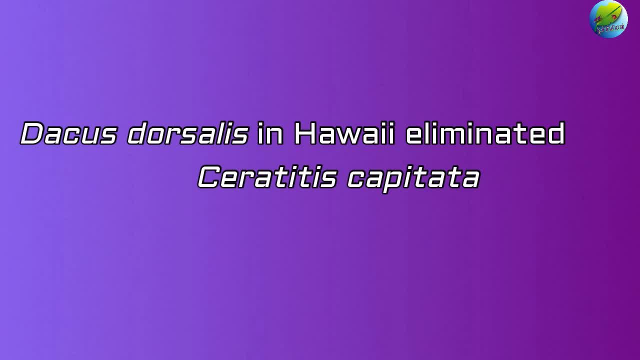 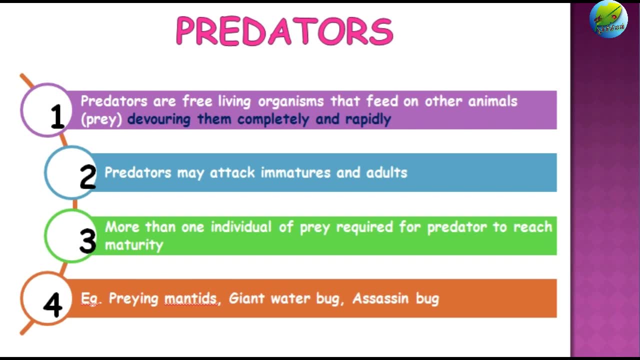 mediterranean fruit fly, that is, the ceratitis capitata. next biotic component that influences the population dynamics is predators and parasites. predators are pre-living organisms that feed on other animals, their prey, devouring them completely and rapidly. predators may attack the immature and the adults. more than one individual of prey required for predator to reach. 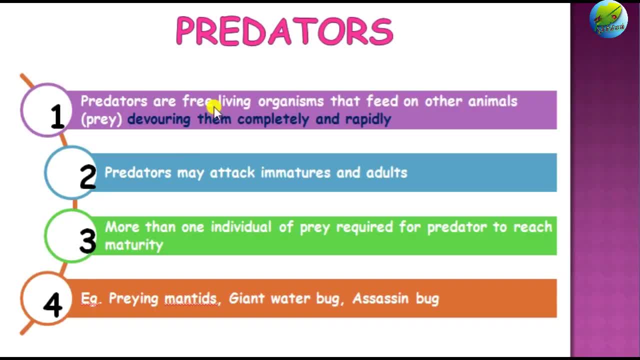 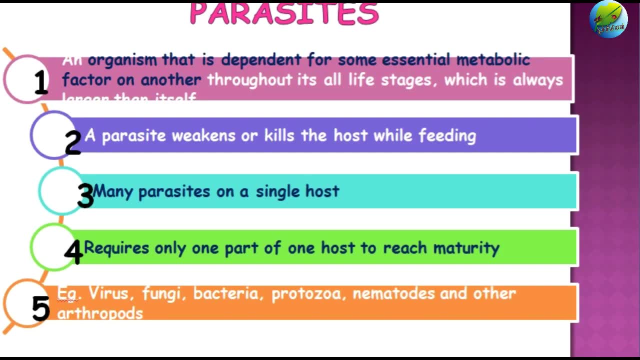 the maturity and the major insect predators are like flying mandates: Jane water bug and the session bugs. next one is the parasites: an organism that is dependent for some essential metabolic factors on another throughout its all life stages, which is always larger than itself. or, as the parasites, a parasite weakens or kill the host while feeding many. 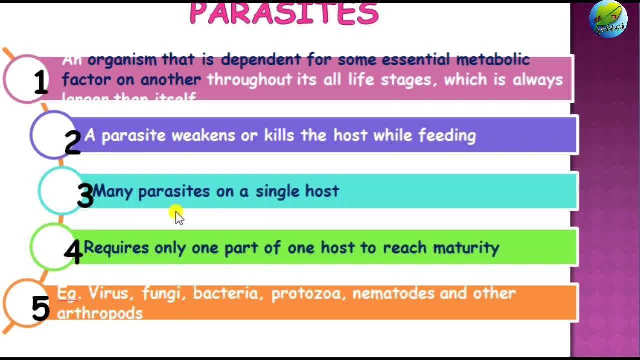 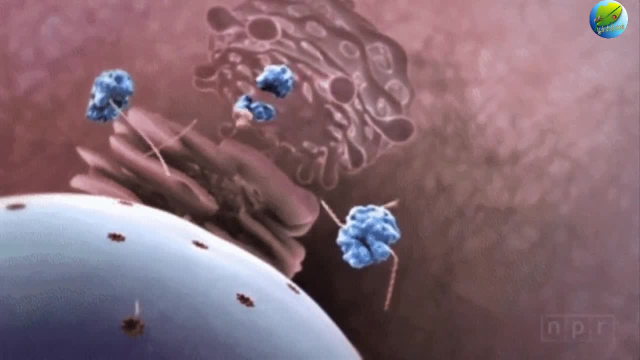 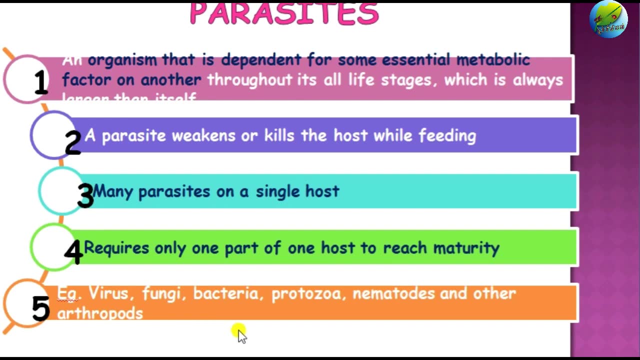 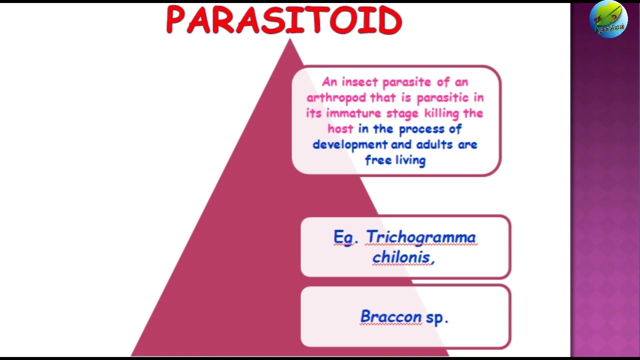 parasites are present in the single host. it requires only one part of a host to reach maturity, which is contradictory with the predators, as they require more than one animal or the more than one insect to complete its life cycle. examples of parasites are virus, fungi, bacteria, protozoa, nematodes and other arthropods. our next biotic factor is the parasitoid. 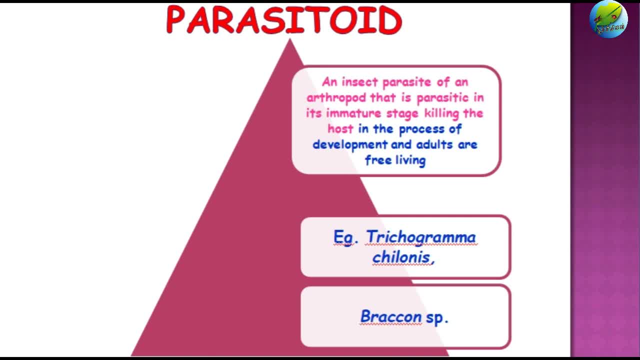 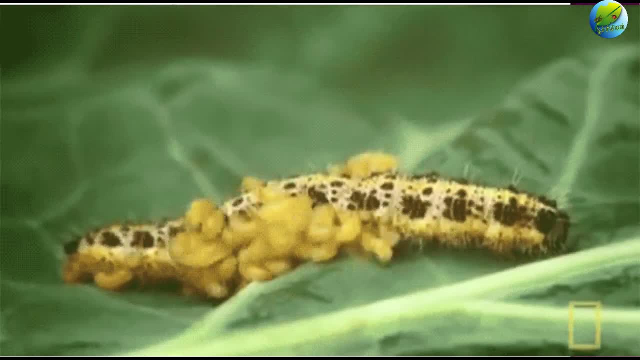 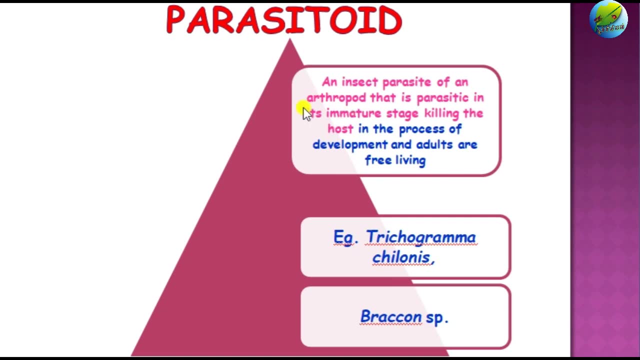 it is an insect parasite of an arthropod that is parasitic in its immature stage, killing the host in the process of development, and the adults are free-living. we must note the point that it is only parasite in its immature stages, as their adults are. 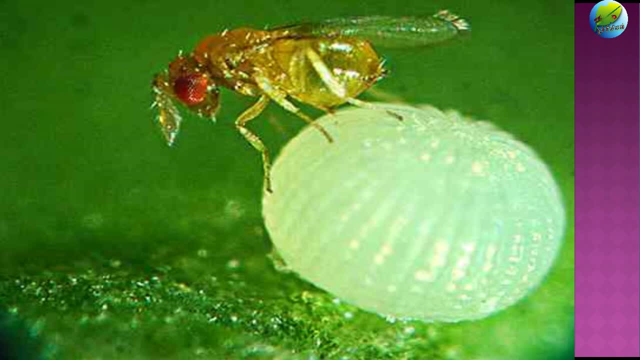 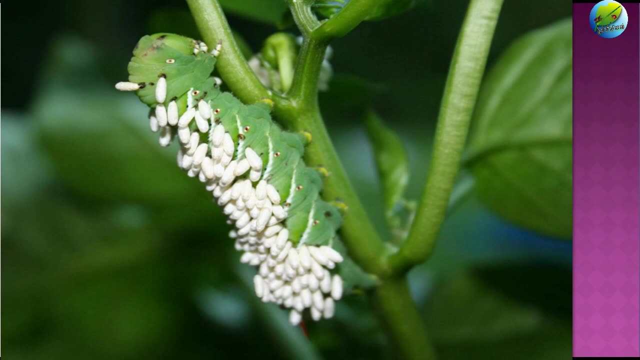 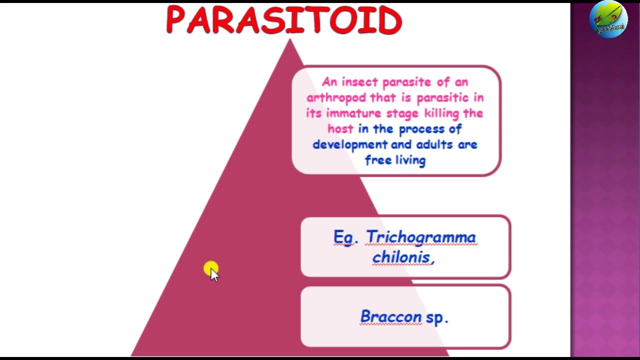 always free living. the example of parasitites are the trichogramma chylonis or the egg parasitite, and the mechanics species, which is the larval parasitoid interaction between predator and prey are different from the parasite host relationship in that the predator 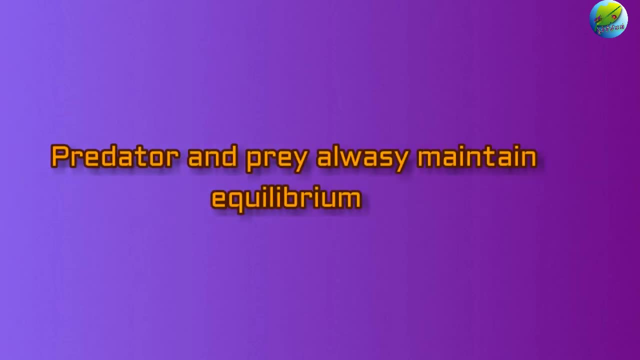 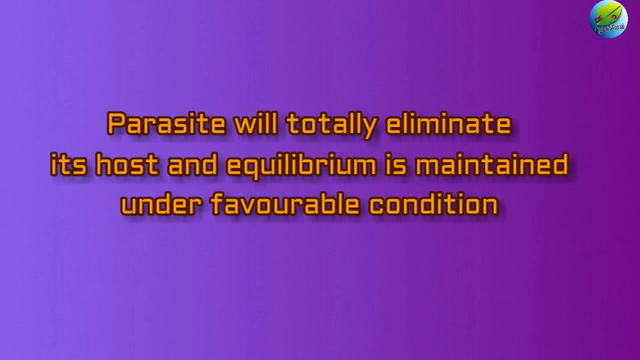 and prey maintain the equilibrium, whereas more dynamic than the parasite and its host. the parasite in general, when the rate parasitism is high, causes death and results in elimination of host. we can set example of the kovat 19 as a parasite, but the predators never. 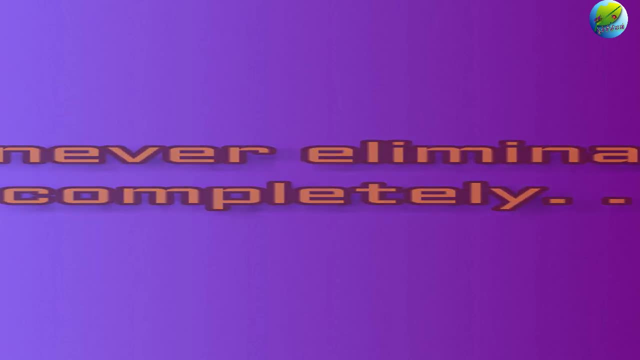 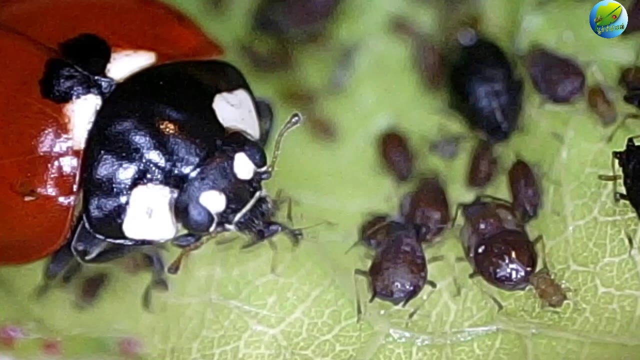 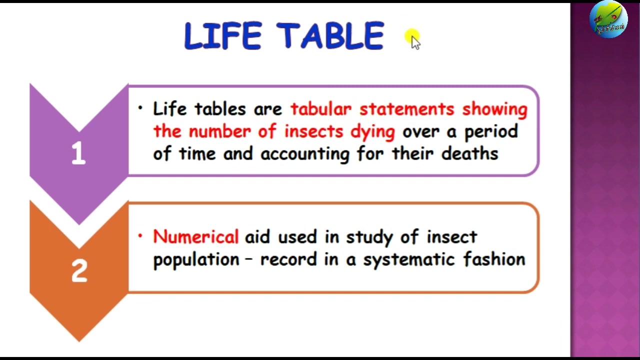 eliminates the prey completely, like if you take the coccinella population. they will feed on the aphids but they will never eliminate the aphid population completely. life table is the numerical aid used in the study of insect population to record in a systematic fashion the number of insects dying over. 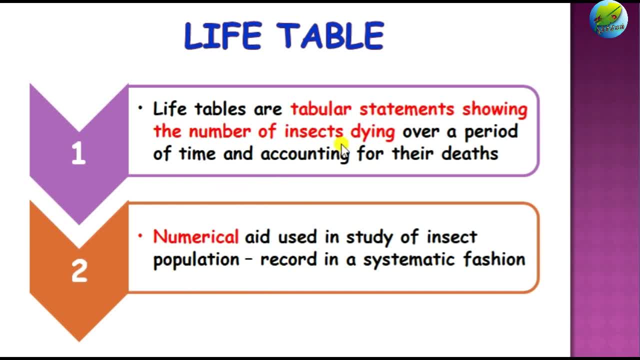 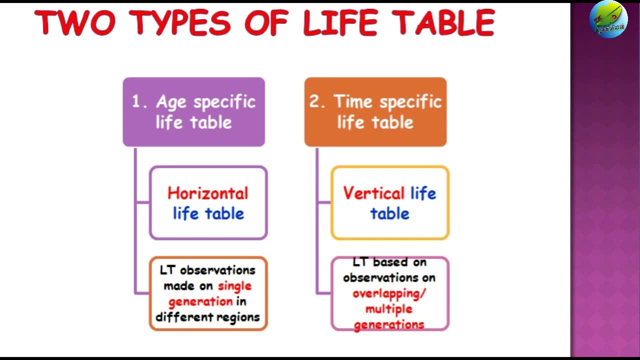 a period of time are often represented in life tables in a tabular form of accounting for deaths. there are two types of life tables, based on their age and the time. in the age-specific life table, the life table, observations are made on the single generation. in the 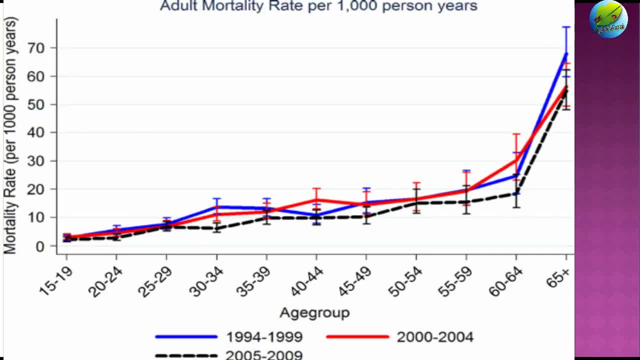 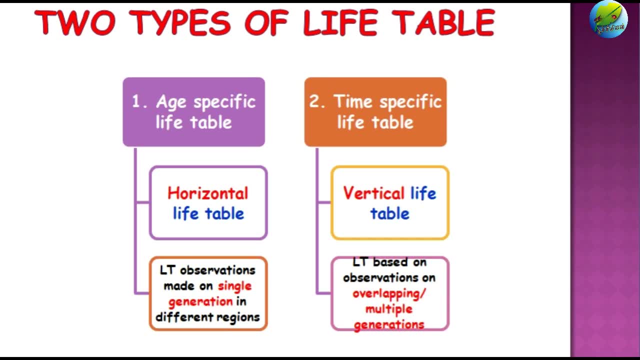 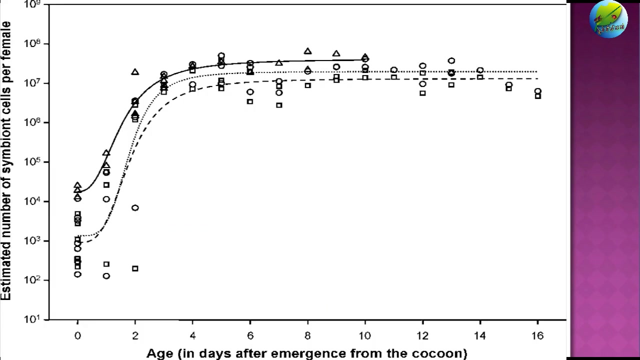 different regions, such as taking observation of the adult population in different regions for only one generation. in the next kind, that is, the time-specific life table, the observation on the life table is made on. the overlapping are the multiple generation in a different time periods, which is otherwise called as the vertical life table, as there is more than. 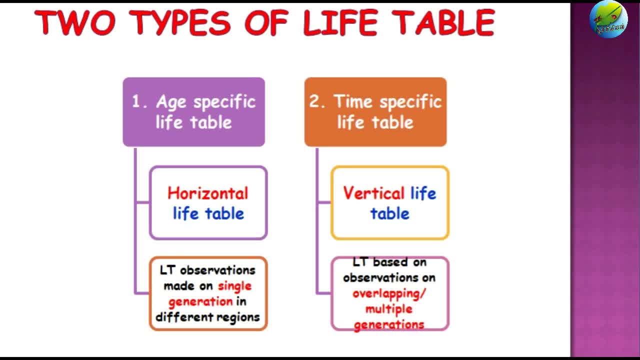 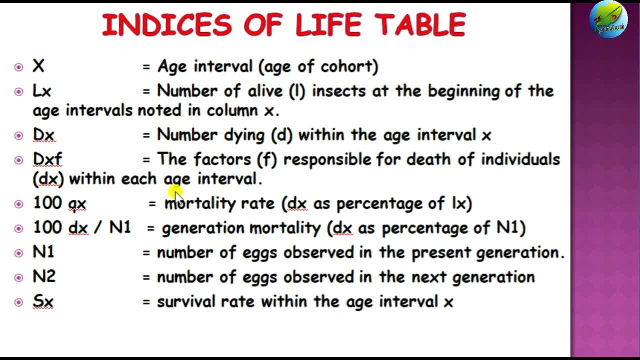 one generations overlapping with each other. these are all the major indices of life table, such as the age interval, number of live insects in the beginning of age interval and the number of dying in the particular age interval and the factors for which is dying, and the number of eggs observed in the present 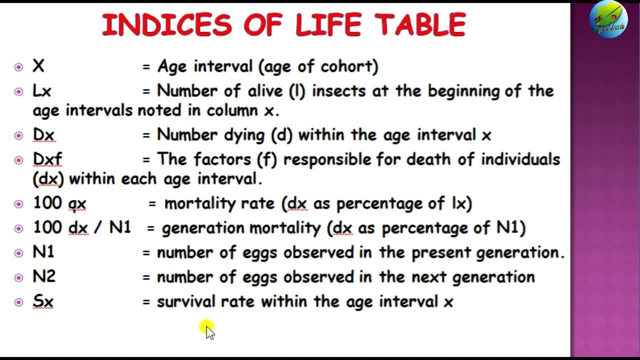 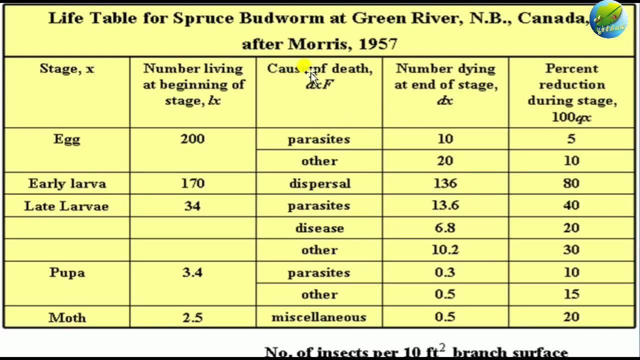 generation and the number of eggs observed in the next generation and the survival rate within the age interval. these are all the indices to form the life table which is denoted in the different letters. here we can see one example in which the life table of the spruce bud form at the Green River is. 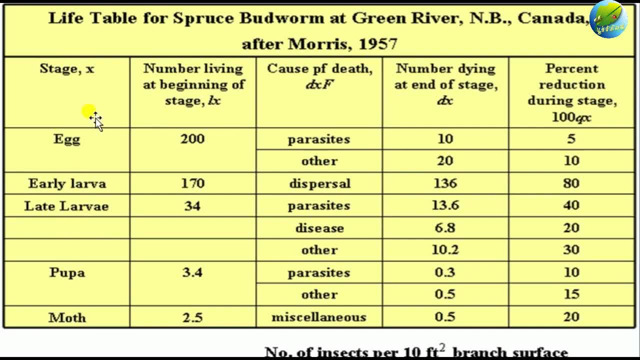 done can see in the X column can see the different age groups, that is, egg, early larvae, late larvae, pupa and Moth. different groups of the age is denoted here and the number of living at the beginning, that is lx, is given here. in case of the yearly larva there was 170 early larvas were alive at the beginning. 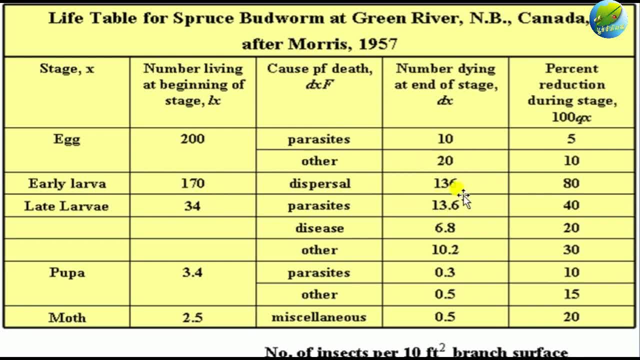 of the, and in the number of dying at the end of the season was 136, which is around 80% of the mortality. the reason was the dispersal. and in the number of living at the beginning was 136, which is around 80% of the mortality. the reason was the dispersal. and if 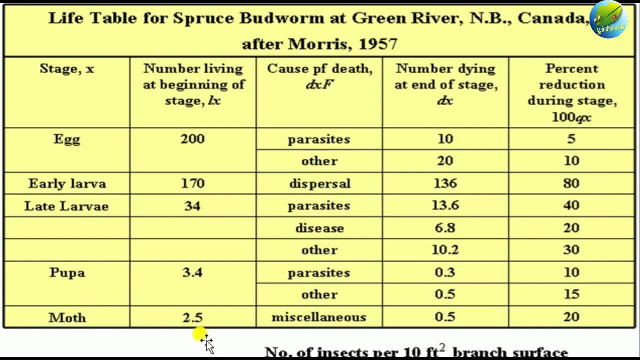 if you see, for math example, there was 2.5 months at the beginning. there is 2.5 is the average number. doesn't mean the two months alive and the of math is death. it is just average number. the number of dying at the end of the stage was 0.5. and the cosmos or any other reasons, such as the 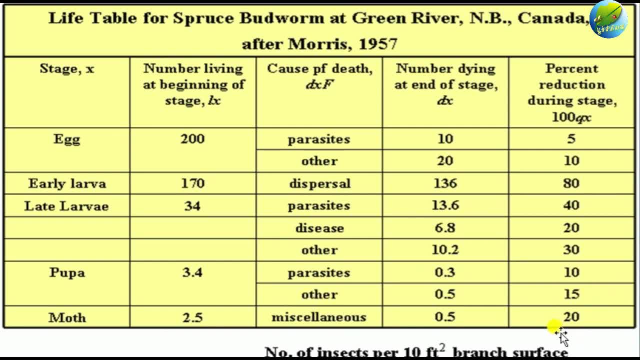 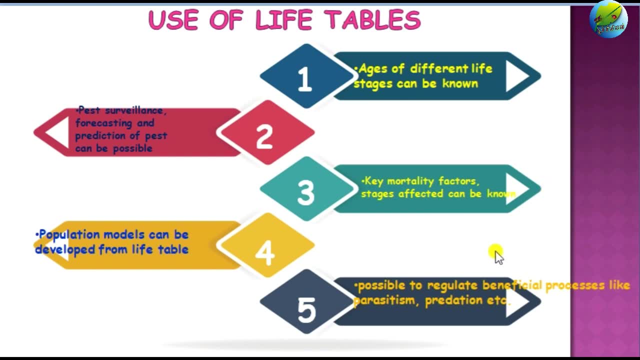 predator and parasites, and the percent reduction during the stage will be the 20 percent. by this way, the life table is being formulated and we can see the uses of them. by the use of life table, we can know the key mortality factor, or what is the main reason the population is dying, and 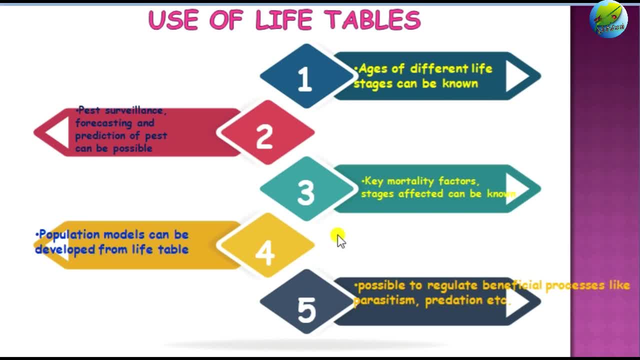 we can also know the reasons, such as the beneficial process, like parasitism, predator or the other factors such as the inter and intraspecific competition can be pinpointed i the population. models can be developed from the life table by having the clear-cut life table. 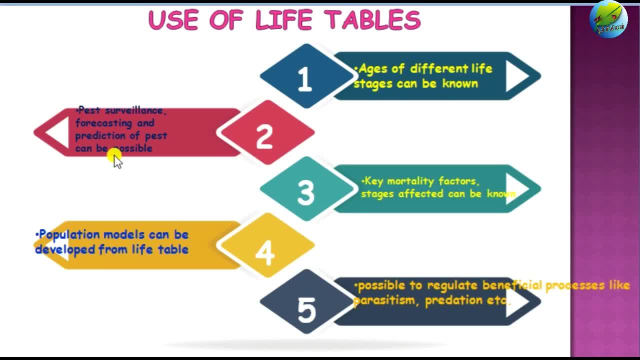 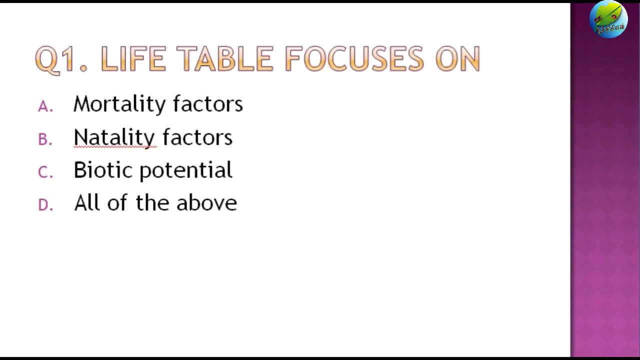 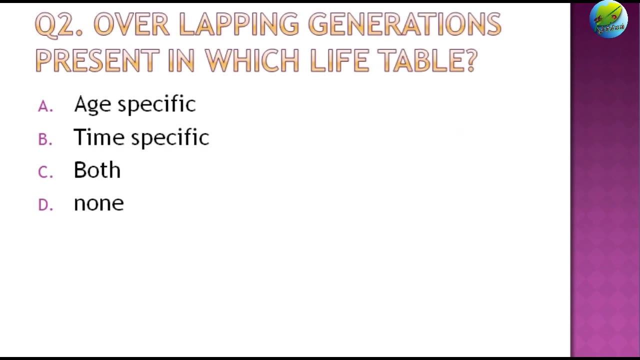 we can form the best surveillance and the forecasting models to help the farmers predict the best population with the available data. okay, let us move on to the question part. question number one: life table focuses on mortality factors, natural defectors, biotic potential or all of the above. overlapping generations present in which life table age specific. 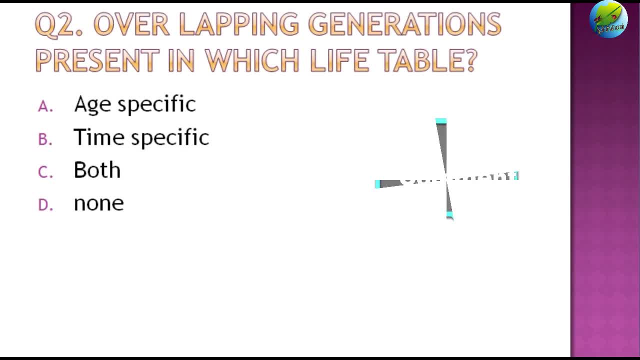 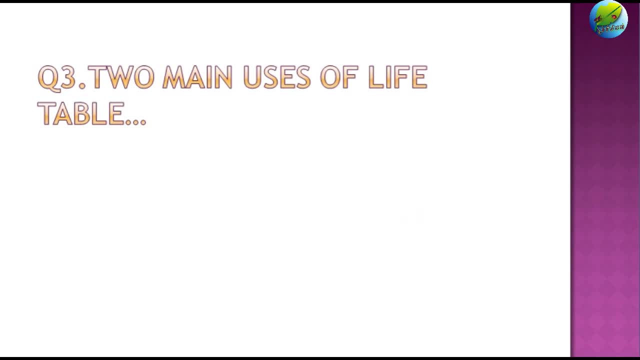 time specific, both of them or none of them? question number three is: write down two main uses of life table. question number four: what is life table darkest does? all is is example far. question number six is: trichogramma is parasite. Querétaro paraceti are non-operable. major difference between parasitized and predator ease. 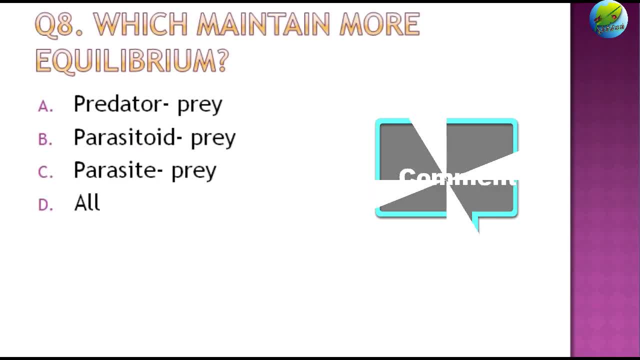 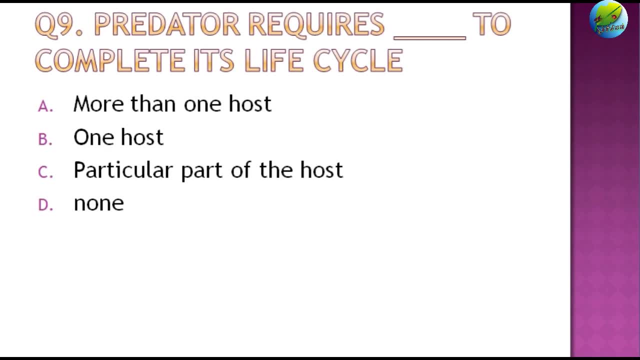 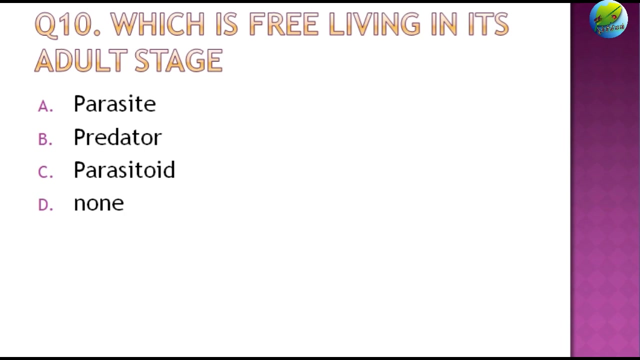 which maintain more equilibrium: predator prey, parasitic prey, parasite prey or all of the above predators, requests dash to complete its life cycle. more than one horse. one horse, particular part of the host or non-operable, which is freely mouthed, living in its adult stage, parasite, predator, parasitoid or none of the above. that's all about. 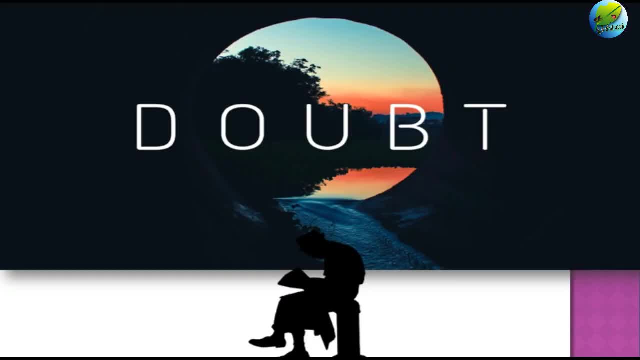 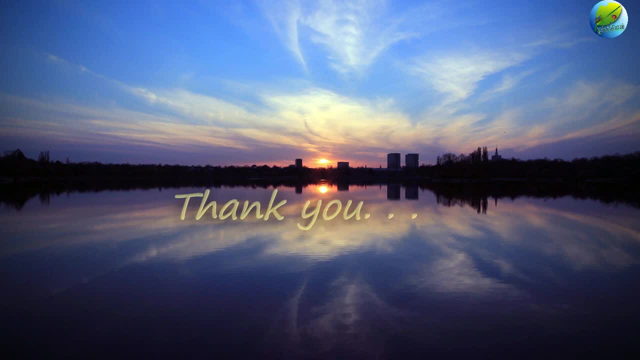 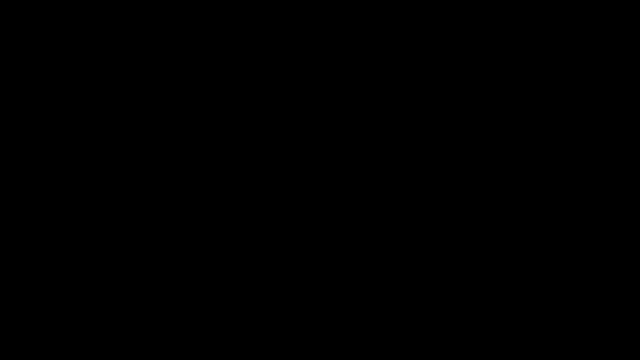 today's class guys. if you have any doubt, put it in the comment. see you in the next class guys. until then, bye.